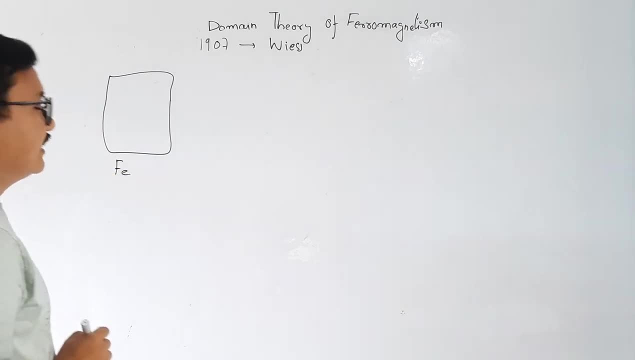 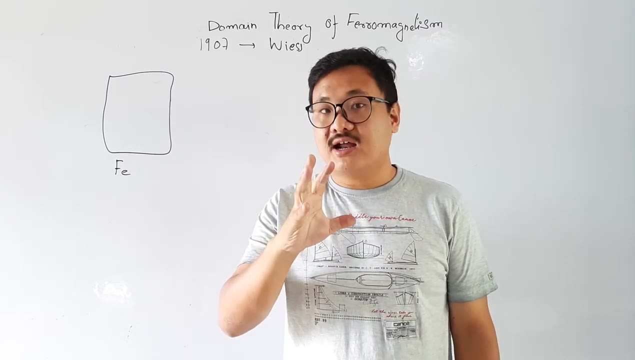 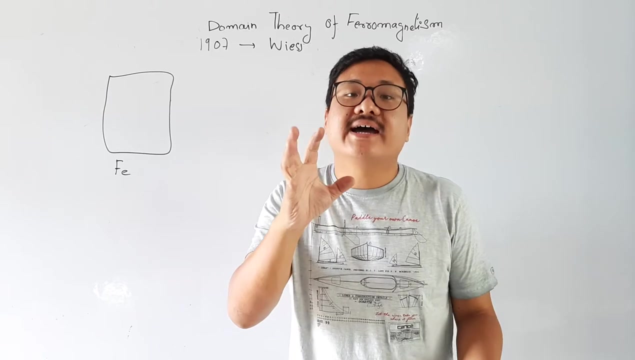 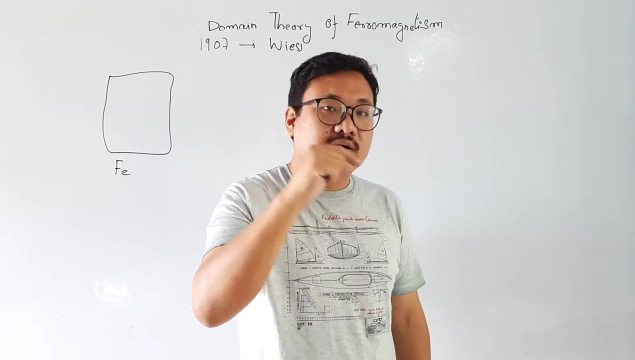 So this is my iron And this is my ferromagnetic material. So in ferromagnetic material there are small, small regions in which the dipole movement are directed in particular direction. In first case we saw that the dipole movements were randomly oriented. 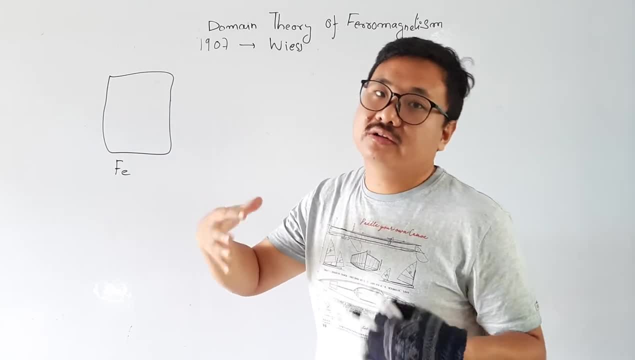 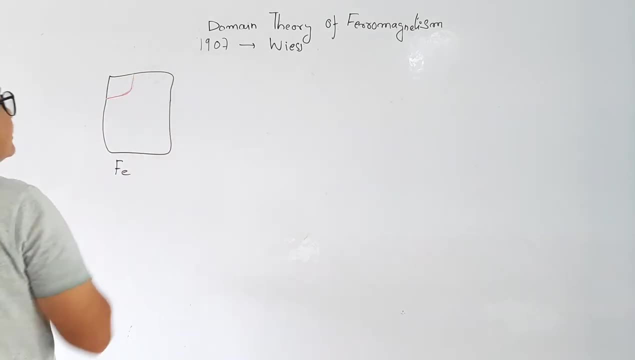 But in ferromagnetic material it is not that scenario. So let us see. So I will consider a small region. So this is my small region And in this region, this is my magnetic dipole movement, or simply the magnetic movement. 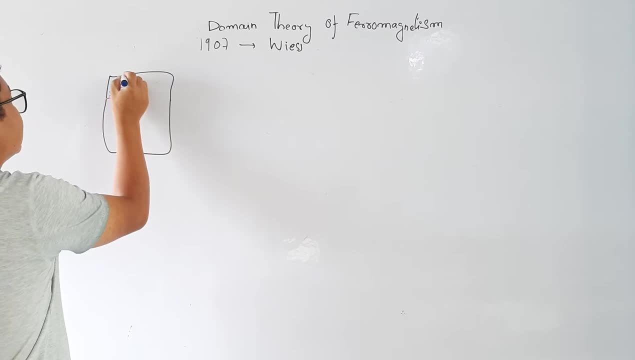 And this is also magnetic movement, and this is also magnetic movement, All are directed in particular direction. So, and this region is called my domain. Similarly, let us consider another domain, Another region, And in this region I will have a magnetic movement in this direction. 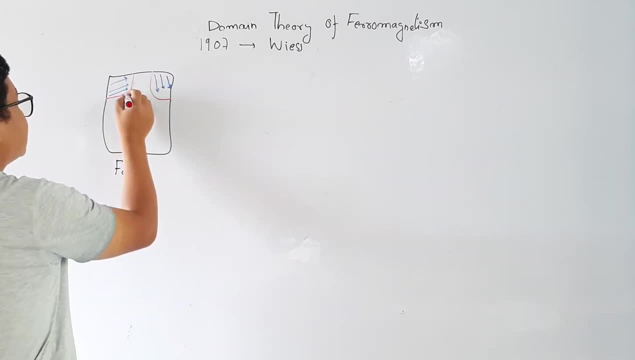 All in a particular direction. Similarly, let us consider this region And in this region. let us have this as my magnetic movement, in this fashion. Now, there are so many regions in which Magnetic movements are directed in same direction. For an example, if we consider this region and in this region, there is a directed movement in this direction. 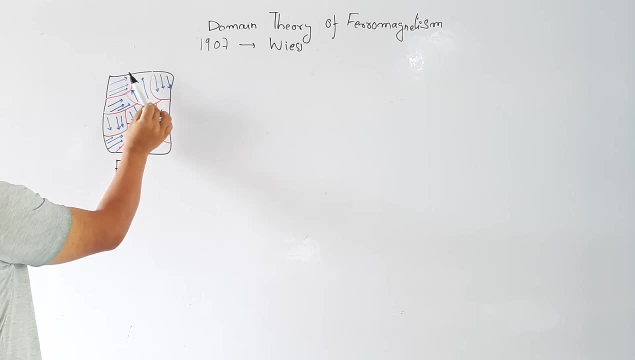 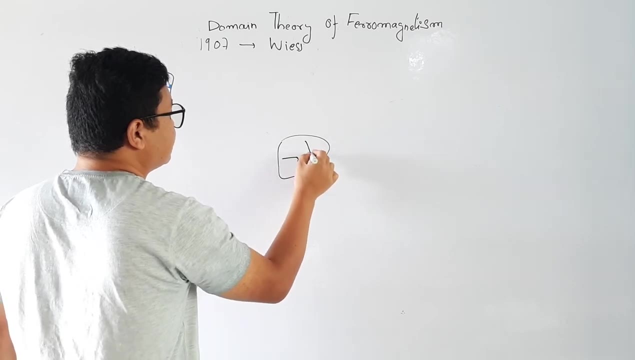 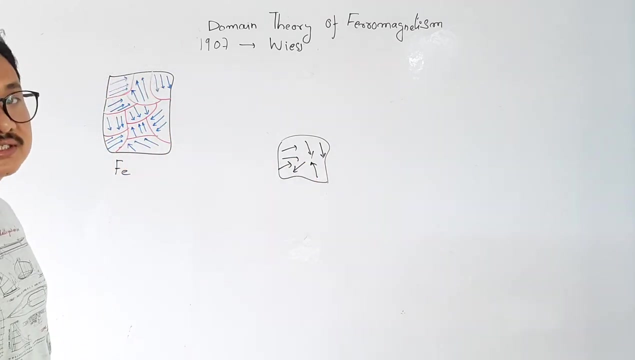 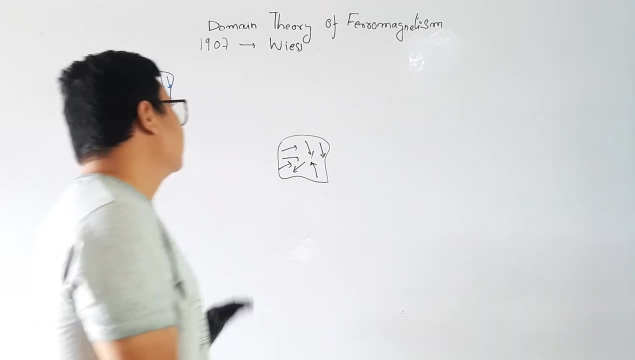 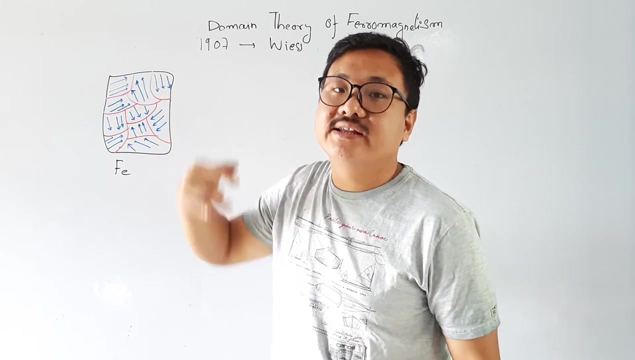 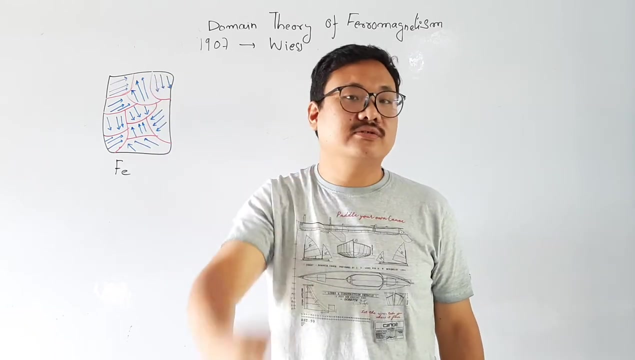 And in this region it is going downward and in this region it is going upward. So in first case we have like this, Okay, Like this randomly oriented, and there were no magnetic regions. Okay, It was like this In first case. but this is the case of ferromagnetic material, and in ferromagnetic material there are small, small region in which there is magnetic movement directed in a particular direction, and that region in which the magnetic movements are directed in a particular direction are called domains. 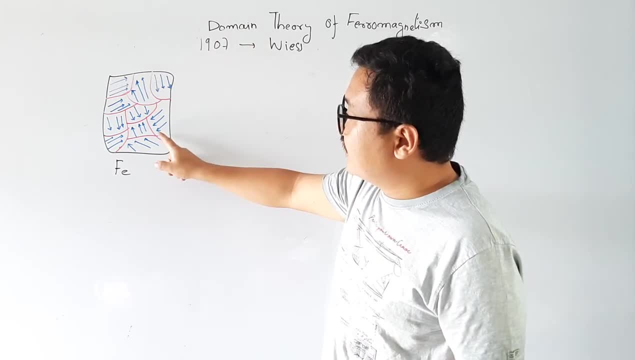 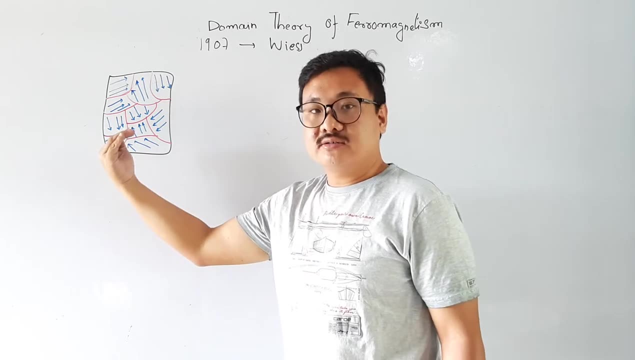 Understood. Okay, So see here, This domain has magnetic movement directed in a particular direction. Okay, This domain has magnetic movement directed in this direction And the domain hasgee directed Moments in this direction. As a whole, the net magnetic field of this material is zero. 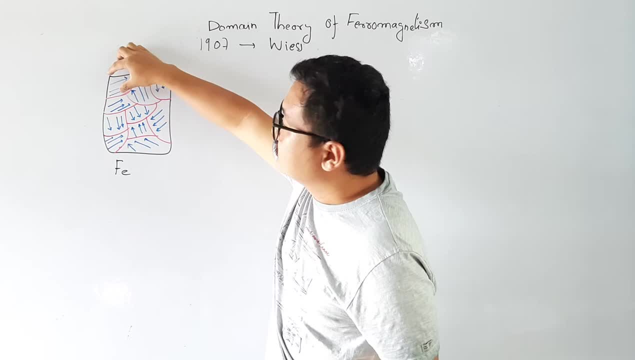 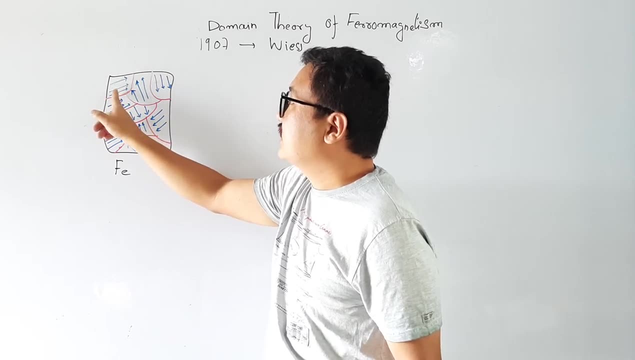 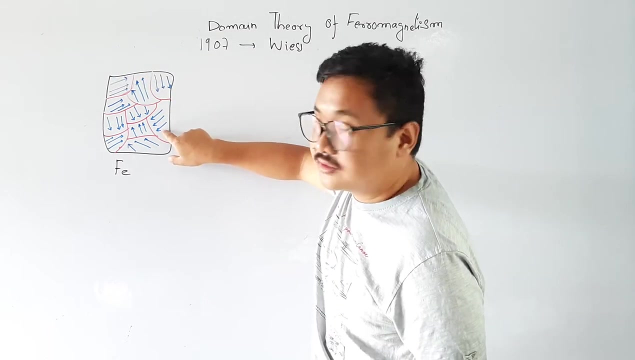 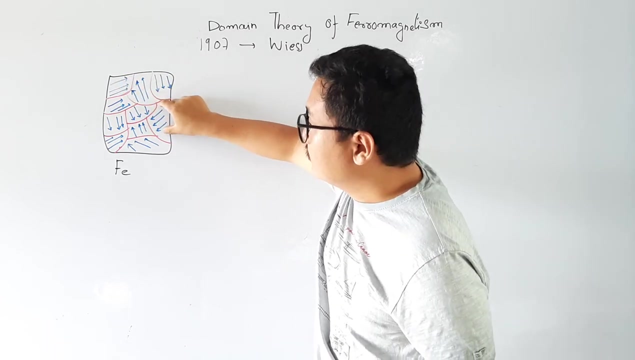 Why? Because this region, this domain, will produce a magnetic field in this direction because of the direction of that movement in particular region. But if you see here This one, Okay, So this one, Speaker 1. Here this is in opposite direction to this one, so this will also produce magnetic field and 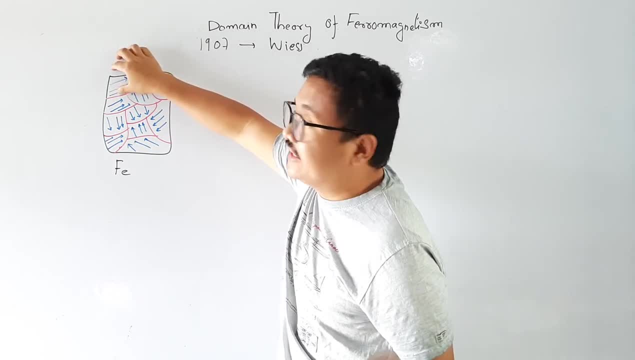 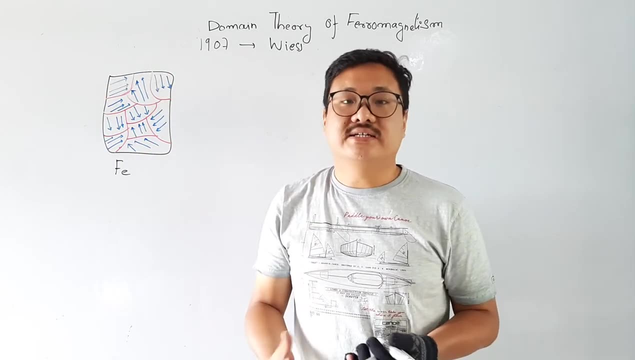 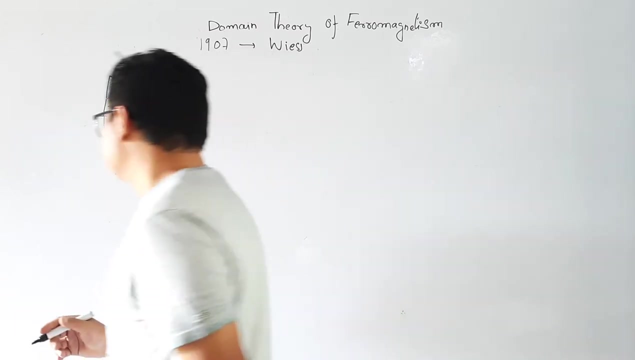 this will also produce magnetic field, but they will produce in opposite direction, one in this direction, other in this direction, so they will cancel the magnetic field of each other. thus the net magnetic field is 0,. ok, So when we say that net magnetic field, net magnetic field is 0 in ferromagnetic material. 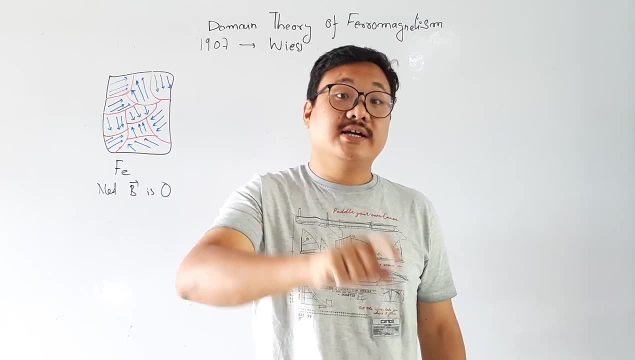 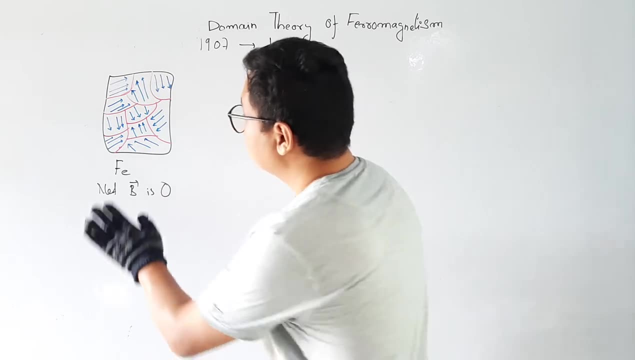 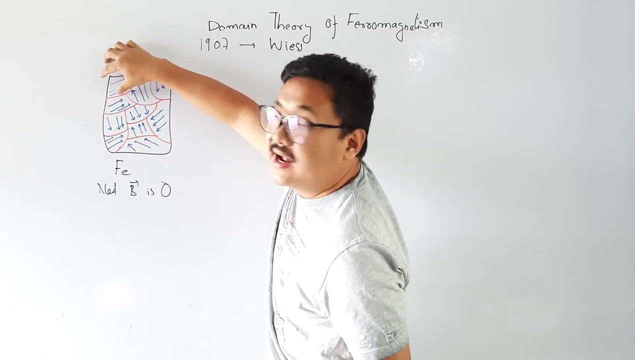 but there is net magnetic field in domains. please remember, net magnetic field is present in the domain. example: if I remove all the domains, this domain, this domain, all the domains removed, then what do I get? I get this domain and in this domain there is a. 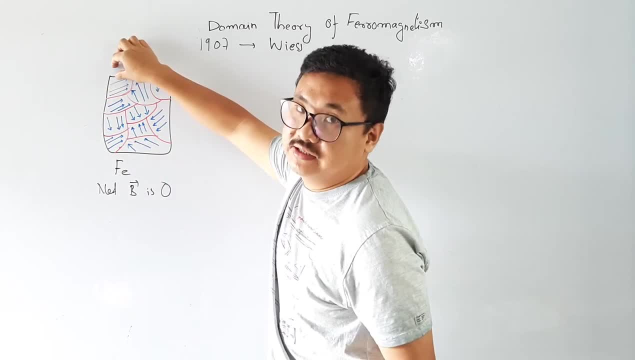 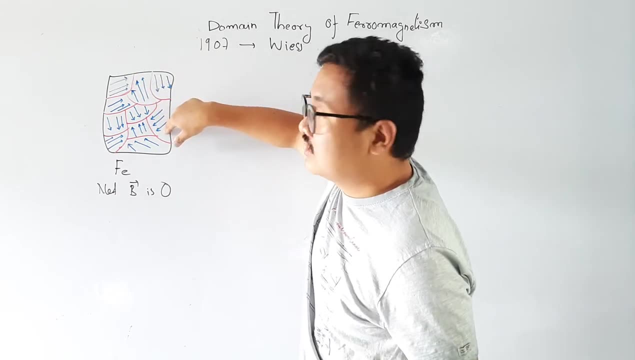 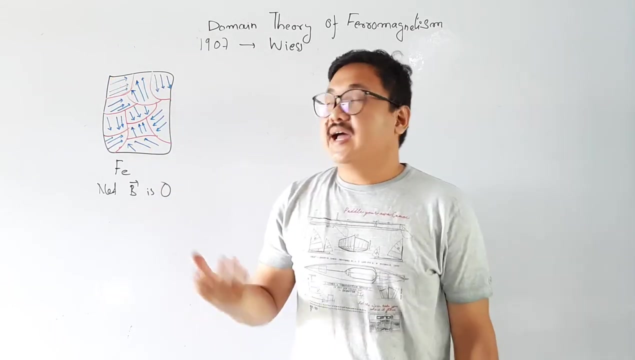 magnetic field. ok, So there is a magnetic field in this direction, so there is net magnetic field. but in this matter, in this element, it has got another domain whose magnetic field is in this direction, which will cancel with this one. so net is 0. and all this small, small region in which 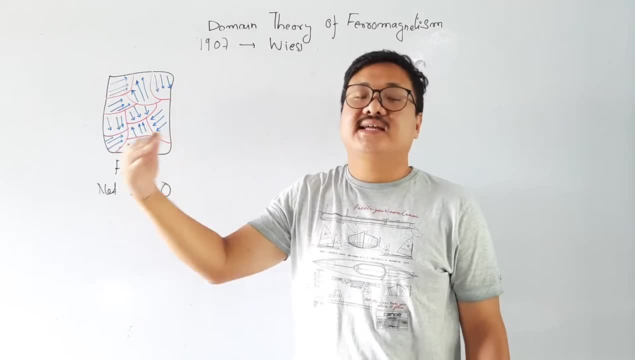 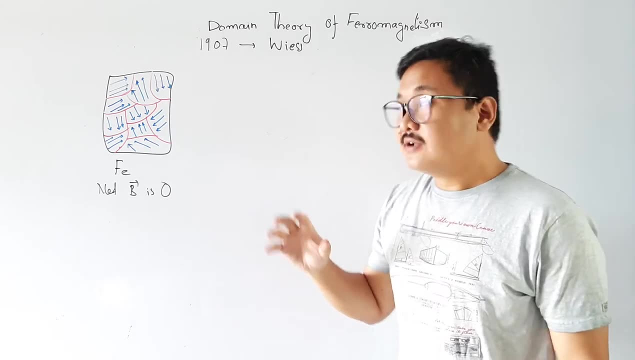 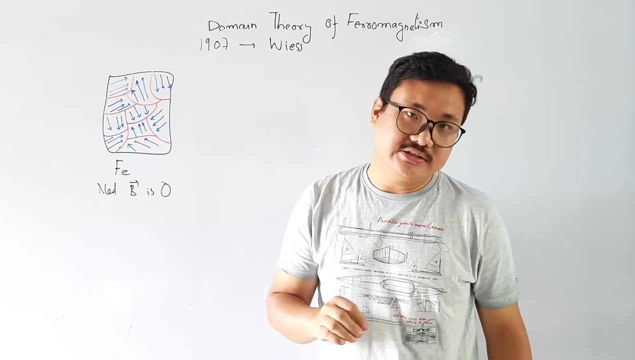 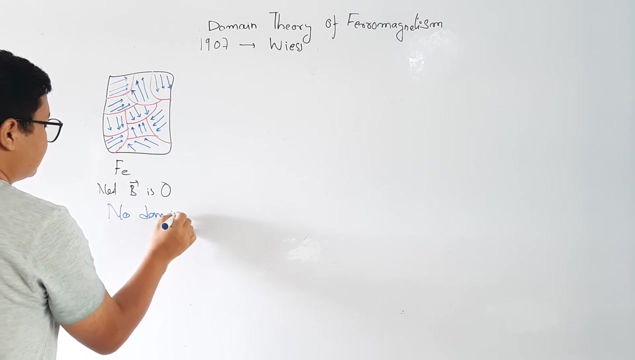 there is magnetic moment directed in a particular direction are called domains. ok, So this is my domain theory And this domain do not exist in diamagnetic and paramagnetic material, ok, So no domain where no domain in para and dia. ok. 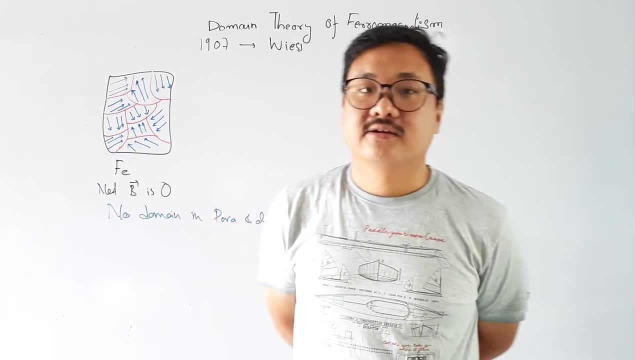 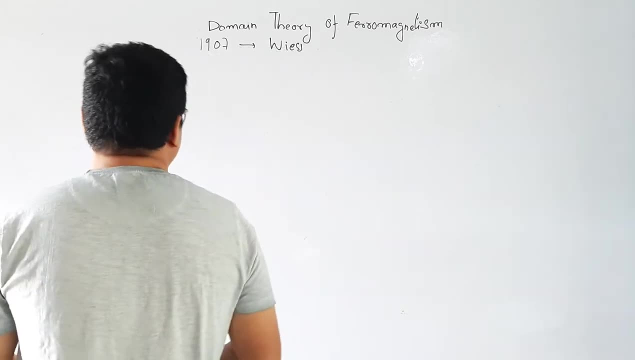 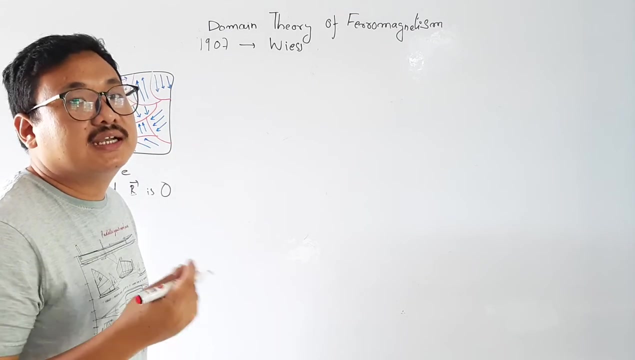 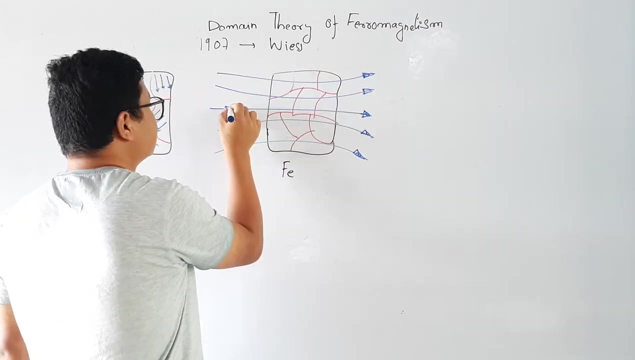 So we only study the domain theory of paramagnetic material. ok, Now, this is case. So whenever I place the, this paramagnetic material, in external magnetic field, let us see what will happen. ok, So let us have this one. so this is again the. so this is external magnetic field. ok, 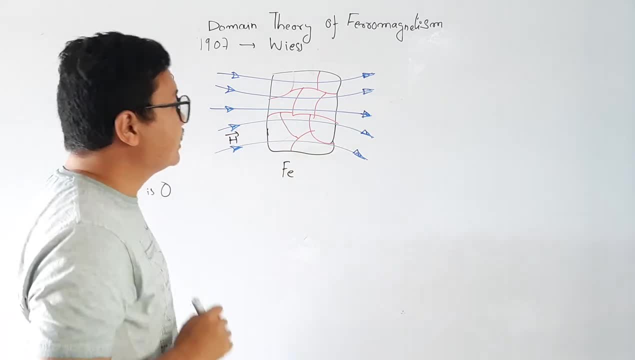 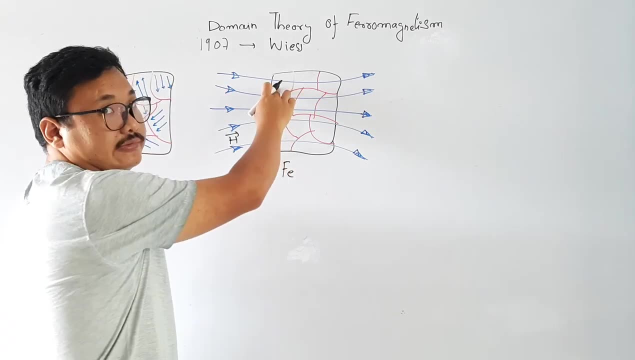 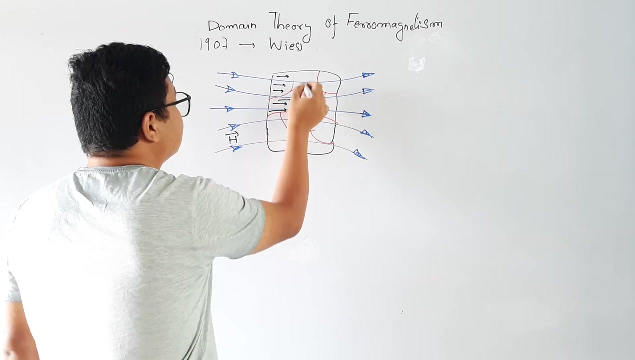 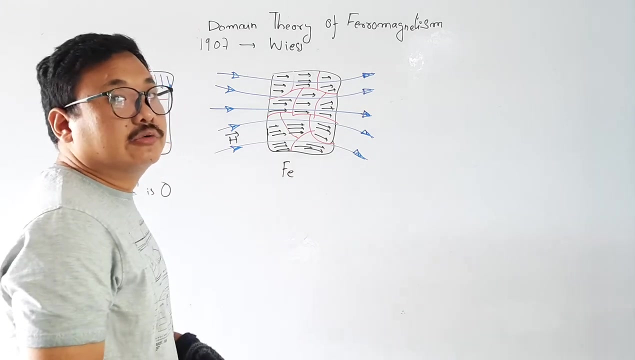 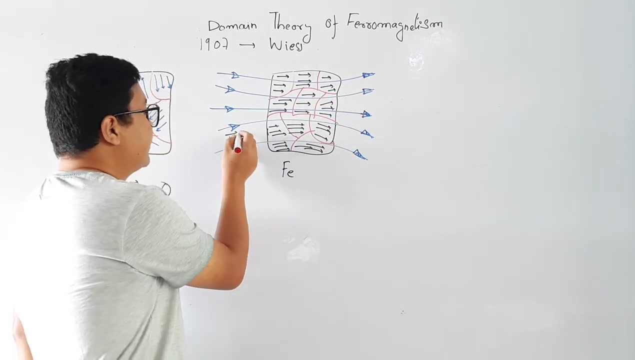 or this is magnetizing field. So we place this in magnetizing field and what will happen to the Diapole moments of this domain? then this will be directed in this direction. Please remember these are very important. ok, So when we place a paramagnetic material in external magnetic field, which is my magnetizing- 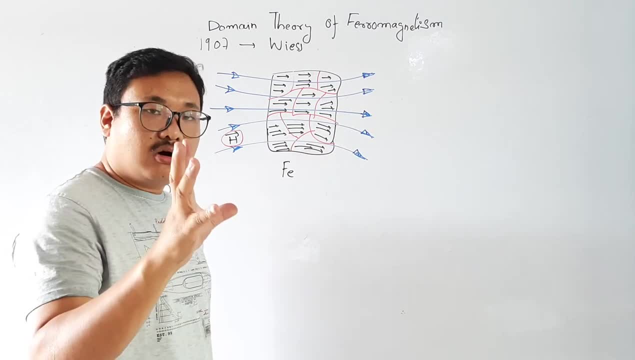 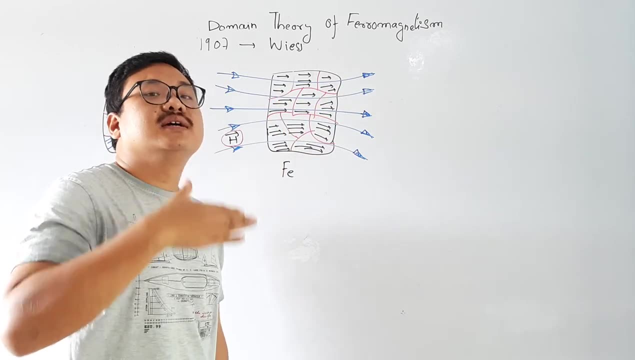 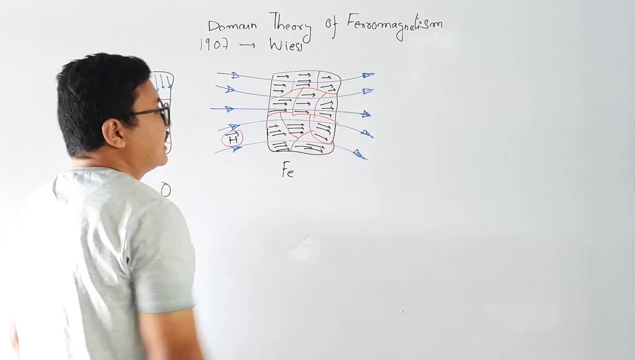 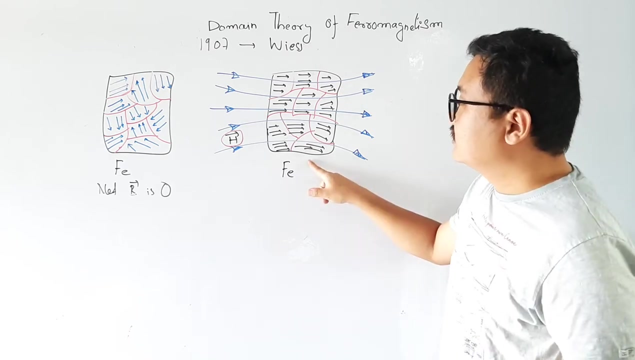 field as vector, then what happens is all the dipole moments of different, different domains align in the same direction of magnetizing field. So these are blue arrows are my magnetizing field and this is my paramagnetic material when placed in external magnetic field. or we can say: this external magnetic field is: 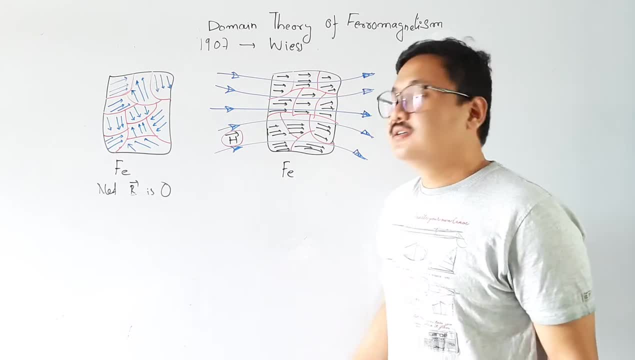 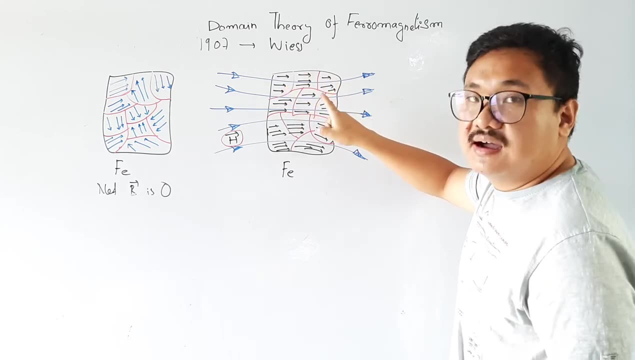 magnetizing field because it is magnetizing the paramagnetic material. So all these, So this is magnetizing material. So all these are magnetizing material. All the dipole movements of all the domains are directed in the direction of external magnetic field. 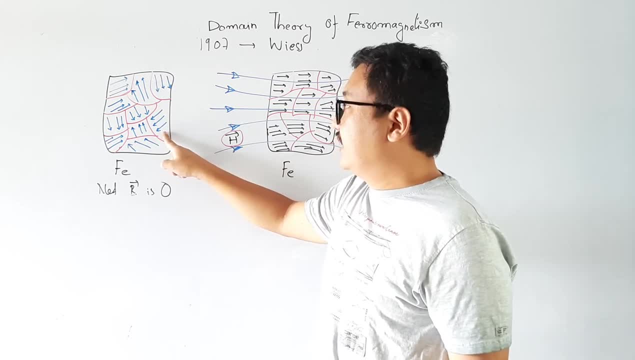 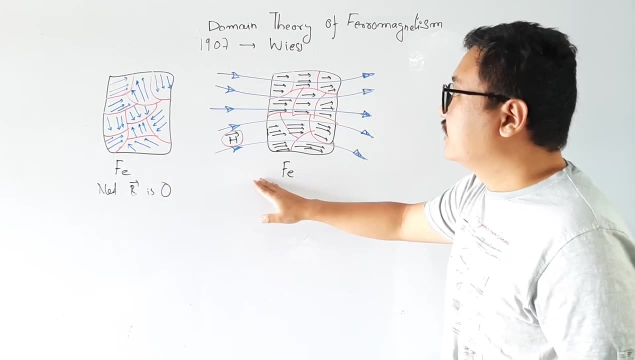 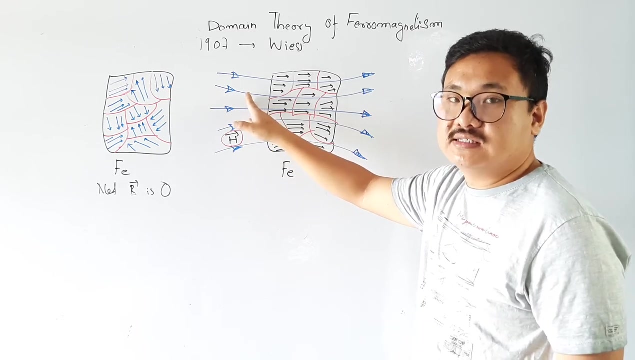 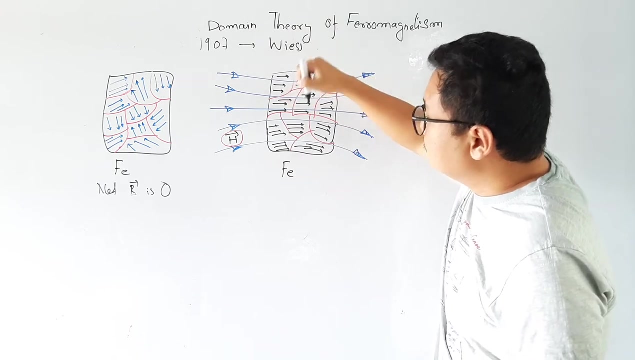 Here domain was there and different direction of dipole movement was there in absence of external magnetic field. Here there is external magnetic field, that is my magnetizing field, and in presence of the magnetizing field the direction of all the magnetic dipoles of the all domains are in the same direction. 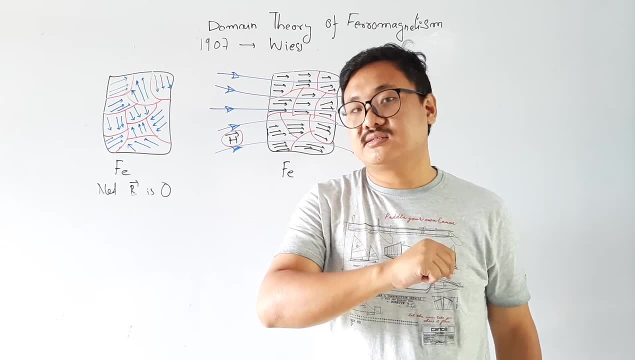 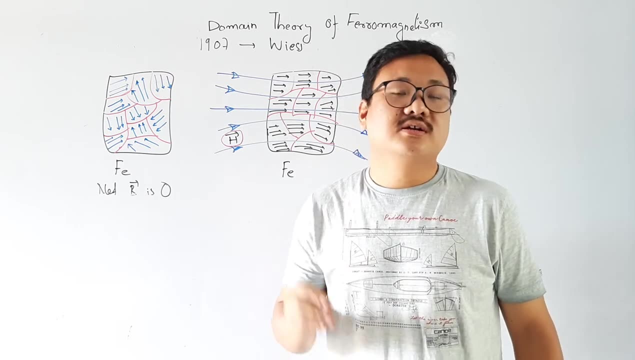 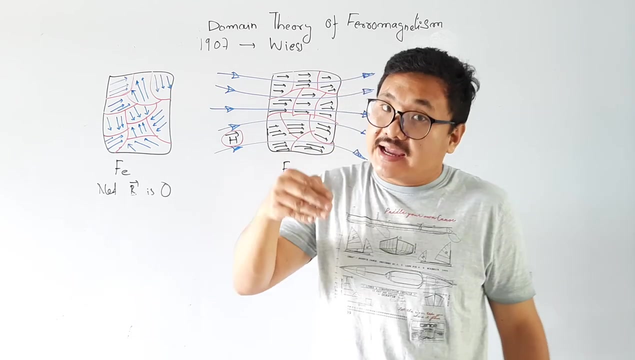 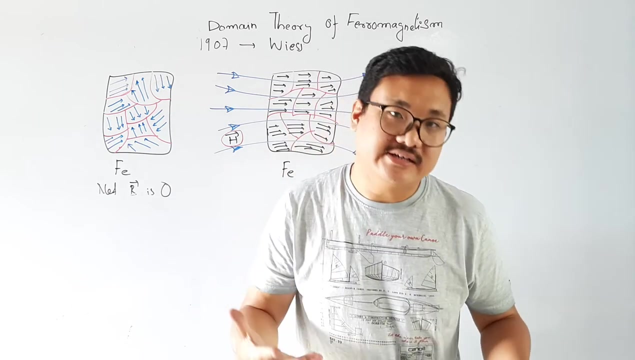 Therefore it get magnetized. The answer is that, if somebody asks you why a ferromagnetic material is easily magnetized, because the dipole movements of domains in ferromagnetic material align itself along the direction of external magnetic field. Thus it get magnetized. 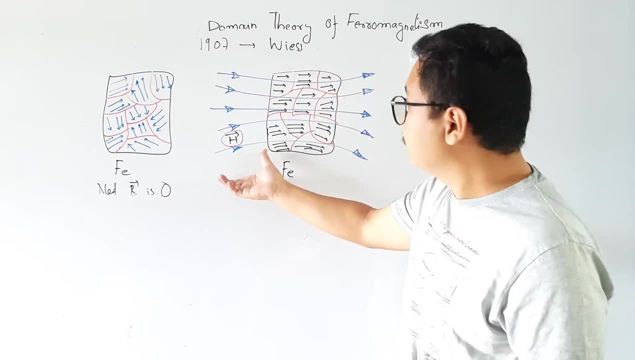 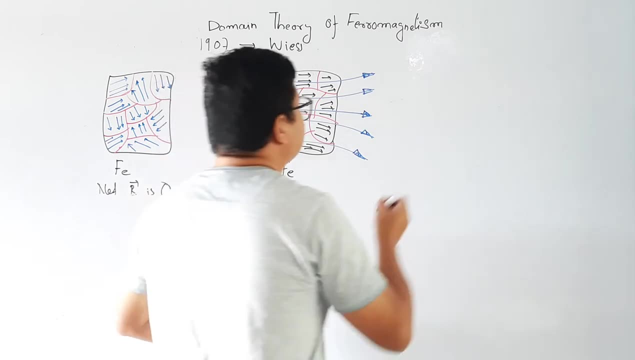 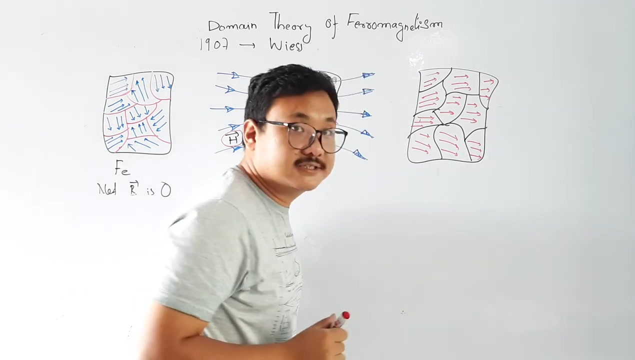 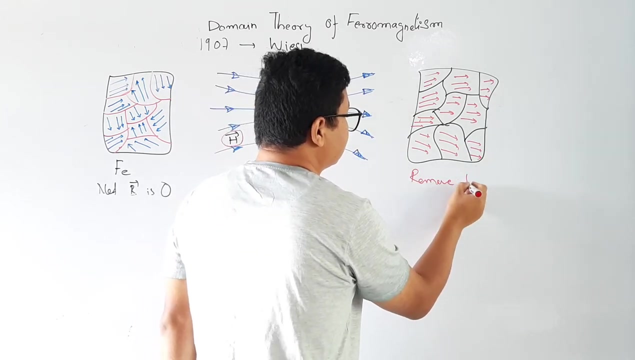 Now let us remove this. Whenever we remove, what do we get? let us see Here: now let us remove the external magnetic field. I have to again consider the same thing. So whenever we remove the external field, We remove magnetizing field, or we can say external magnetic field. 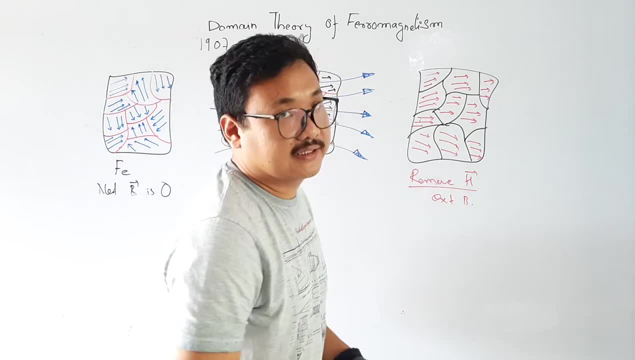 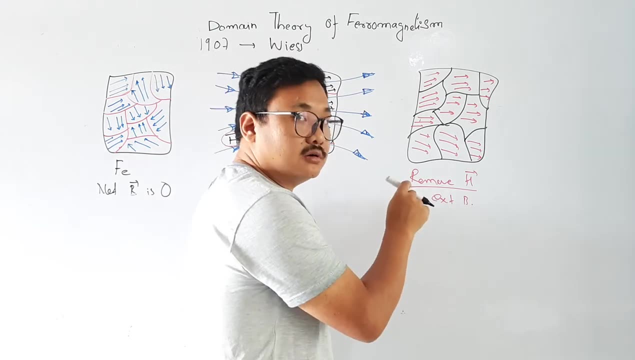 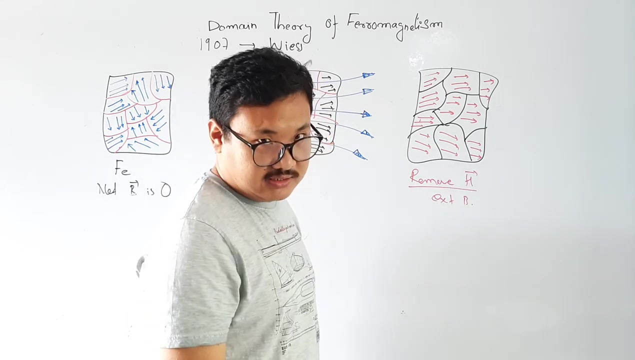 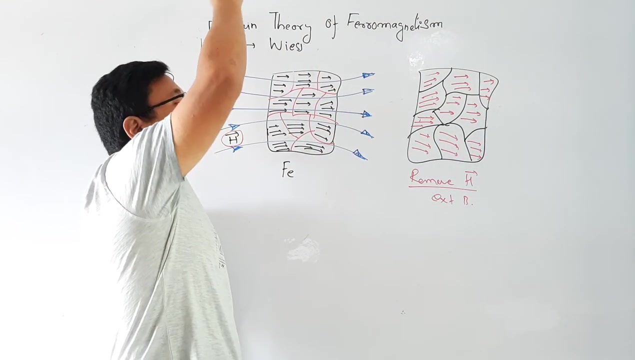 External magnetic field. then what do we see that? we see that the dipole movements of the domains are also in the same fashion. Now, even after the removal of the magnetic field, the dipole movements in all this small, small region which is my domain are still in the same direction. 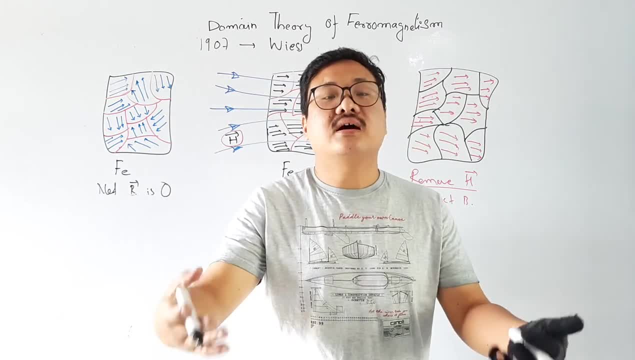 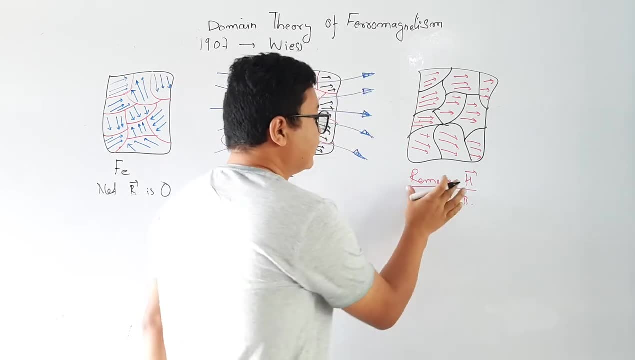 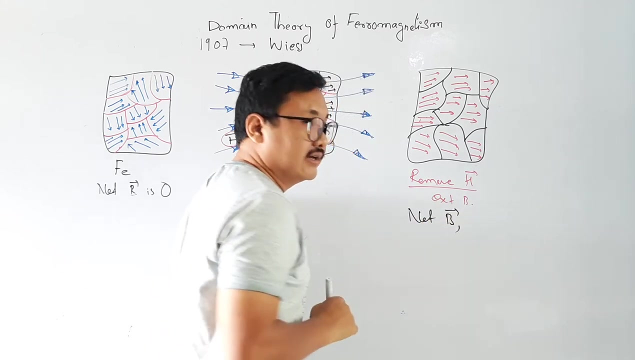 What does this mean, then? It means that, Even after the removal of external magnetic field, there is net magnetic field. Whenever there is removal of external magnetic field, there is net magnetic field. And why? Because, very important, because after the removal of magnetizing field, which is this one, 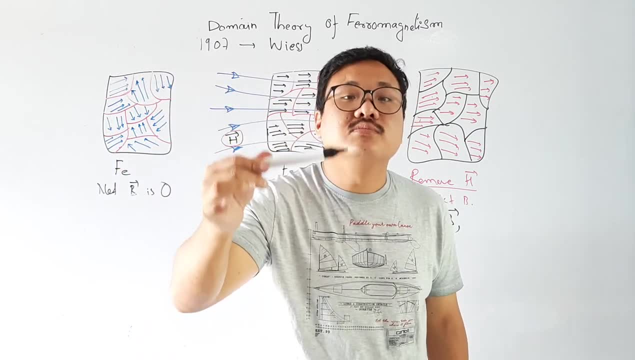 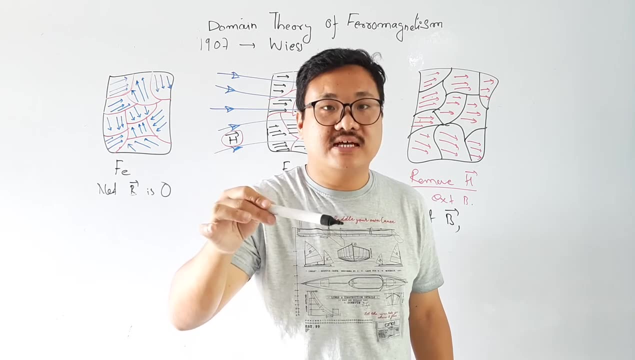 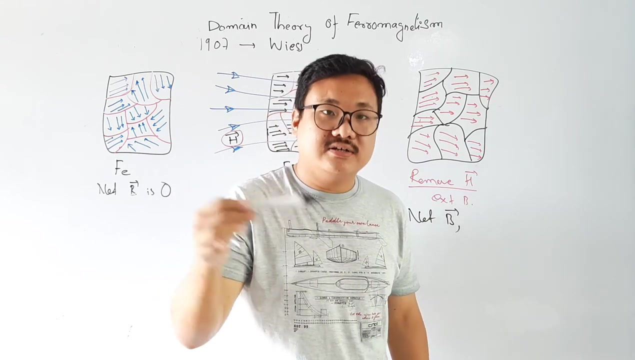 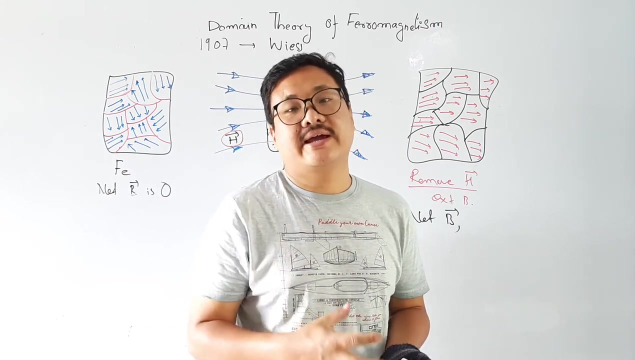 The direction of the dipole movements of the domains. The different different domains are still aligning themselves in the same direction. That is why they will have a net magnetic field in that direction. So even after the removal of external magnetic field, there exist a net magnetic field. 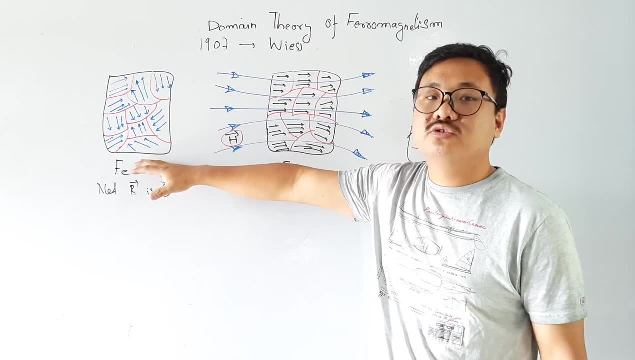 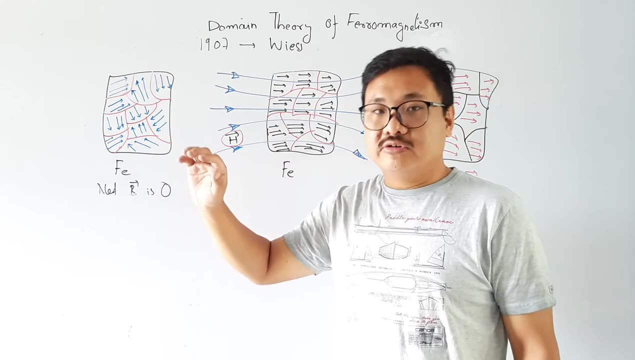 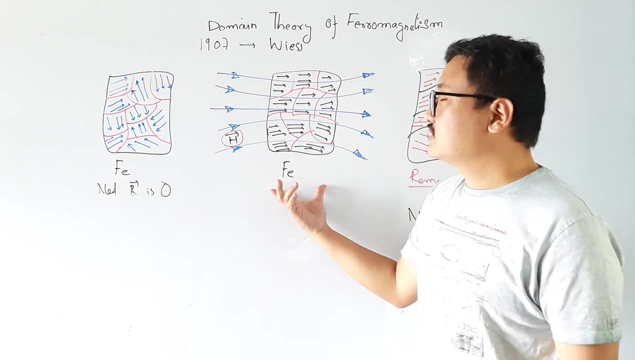 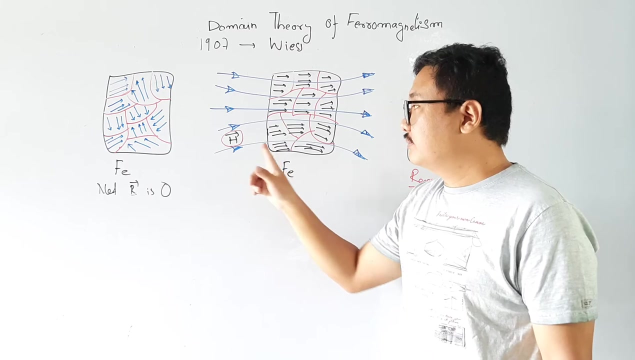 So we got the three phases. One: there was no magnetic field, I mean external magnetic field was absent, And there was domain Domains means small, small region in which there are net magnetic movements directed in particular direction, And we place the same magnetic material, that is, ferromagnetic material, in an external or magnetizing field. 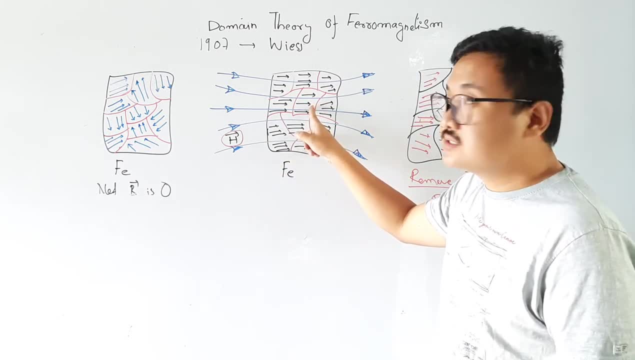 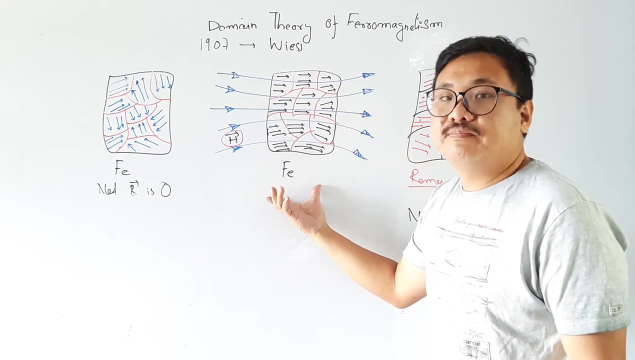 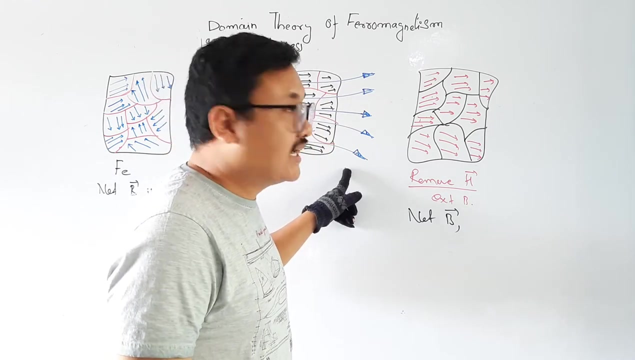 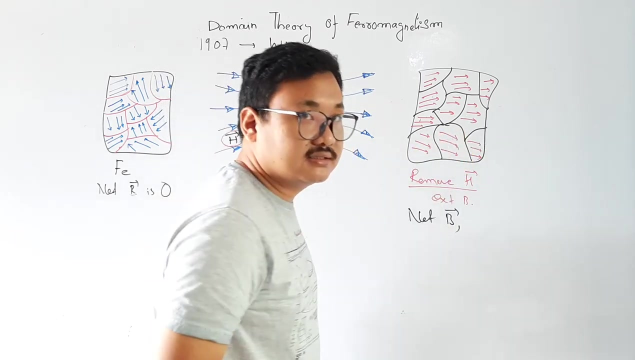 The domain and the magnetic movements of that domain align themselves in the direction of external magnetic field And it got magnetized. Now, after the removal of the external magnetic field, We saw that the direction of magnetic movements are still aligning themselves, are still in the same direction. 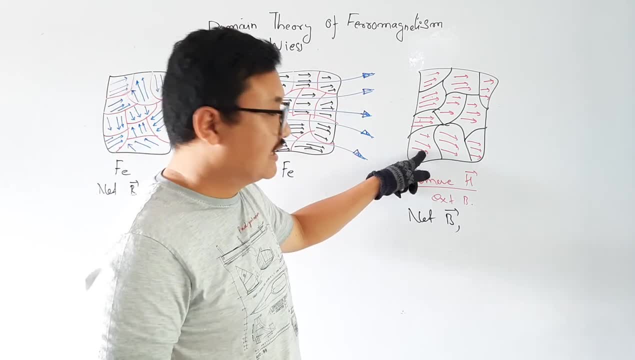 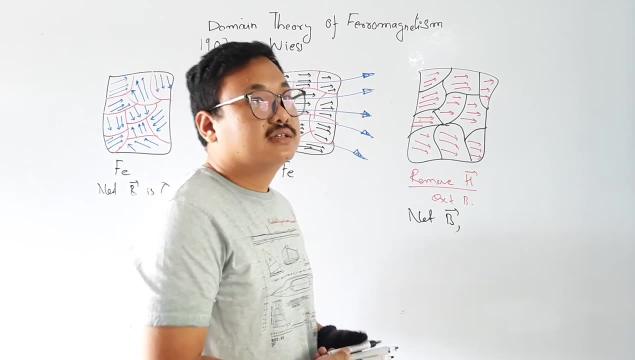 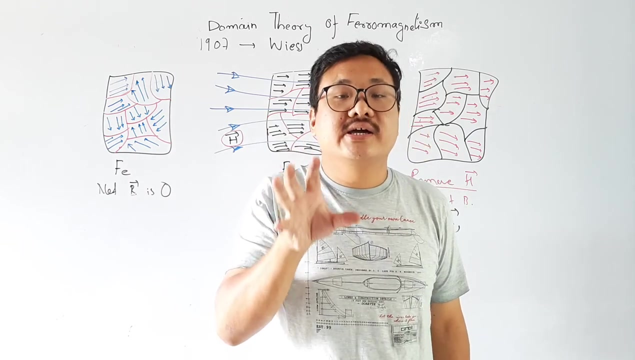 Unlike this one. So here there we get the net magnetic field. Because after the even removal of magnetic field, There is the direction of magnetic movements. The magnetic movements are in the same direction. That is the reason why a ferromagnetic material get magnetized.